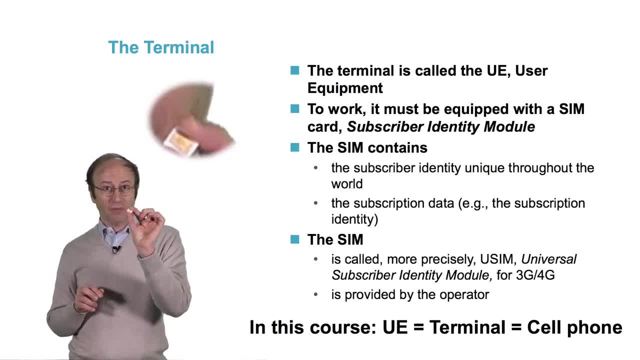 or Subscriber Identity Module, contains the subscriber identity, unique throughout the world. It also contains data about the subscription. In France, the SIM card is property of the operator. This card is called a USIM or Universal Subscriber Identity Module, in 3G or 4G. 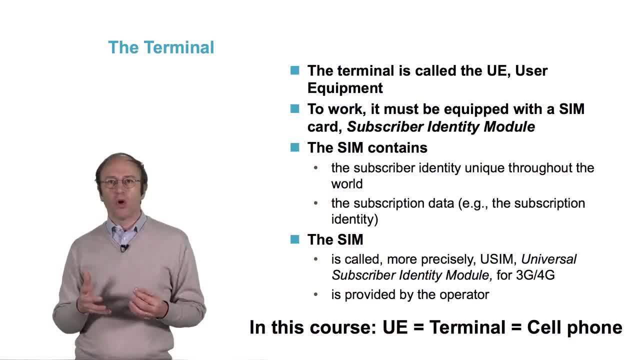 However, in the videos we use the acronym SIM because it is simpler and often used indifferently for 2G, 3G and 4G. The SIM card is found in equipment such as a smartphone, but it can also be found in a 4G key or a router that I can connect to my laptop. 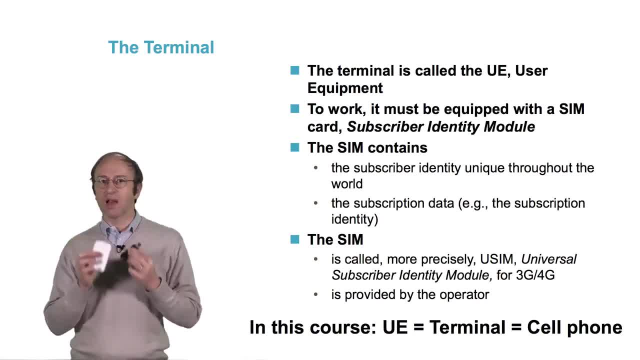 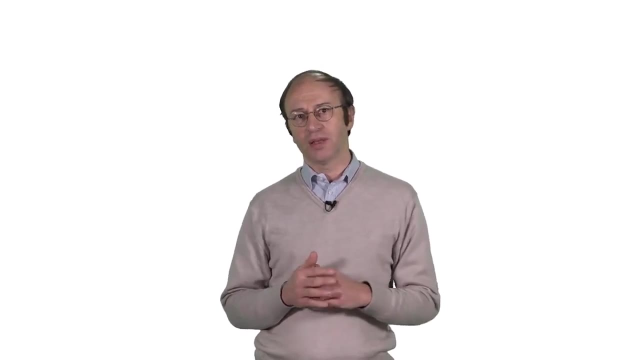 In order to have mobile internet access on my laptop. In this course, we are not going to differentiate between types of terminals. All terminals will be treated identically. Obviously, the network is not limited to that. If we walk in the street, we see antennas on the roofs of buildings. 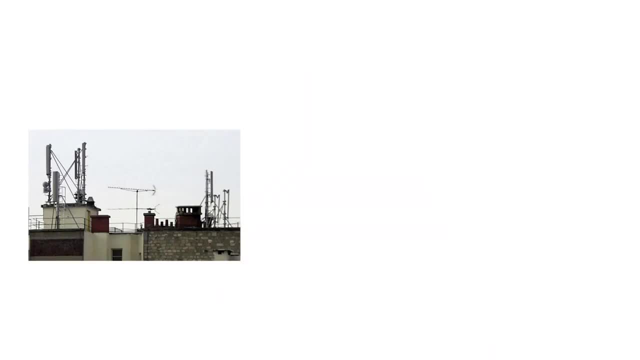 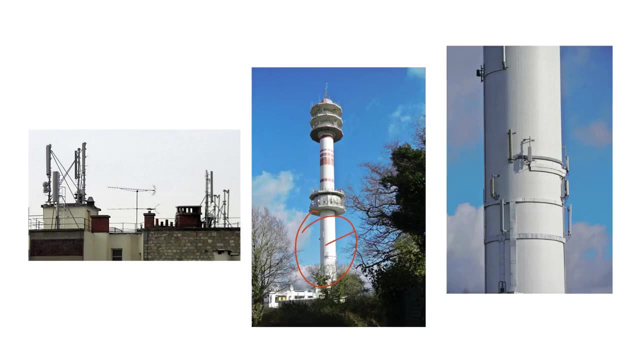 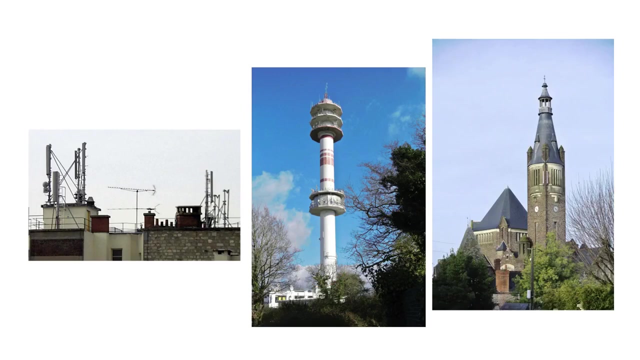 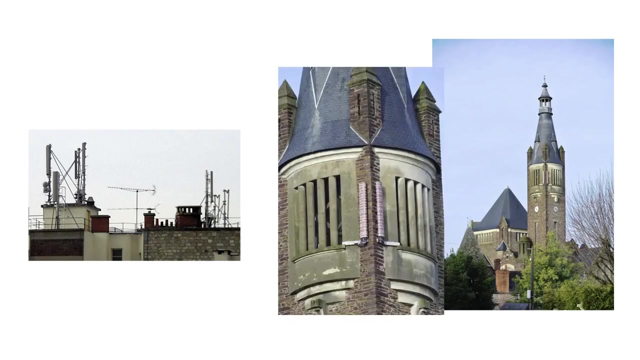 like this one or on towers like this one. With a zoom we can clearly see the antennas. In some cases it's a bit more difficult to see, but here we have an antenna on this church. If we zoom in we can clearly see the antennas on the bell. 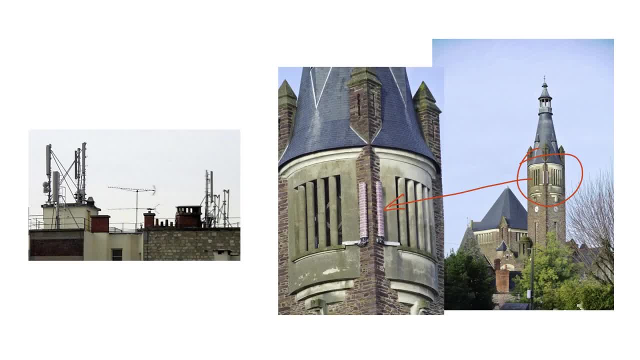 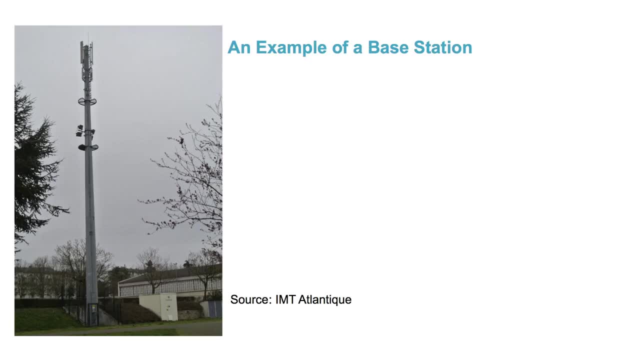 If we pay very close attention, in some cases, what we see is this antennas on a mast and beside it a technical cabinet. What we see are antennas, In other words, a radiating device that transforms high-frequency alternating current. 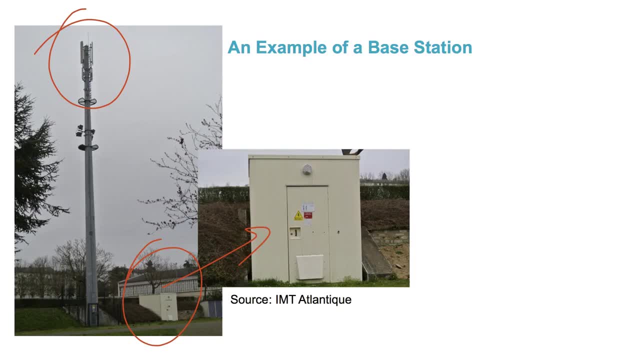 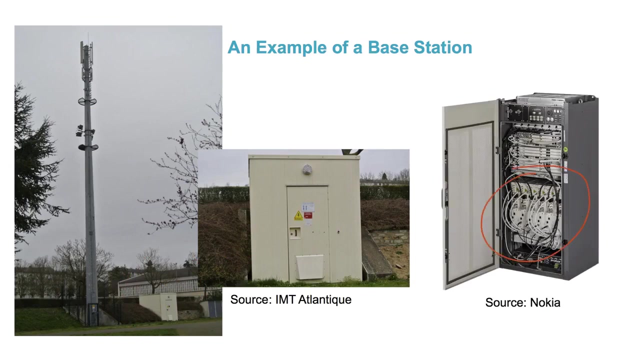 In other words, a radiating device that transforms high-frequency alternating current into electromagnetic waves or the other way around. In the technical cabinet, if we open the door, we see a set of transceivers that will enable radio transmission between the terminal, which is also a transceiver, and the network. 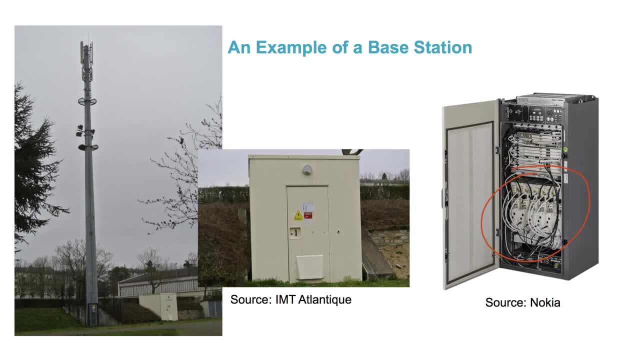 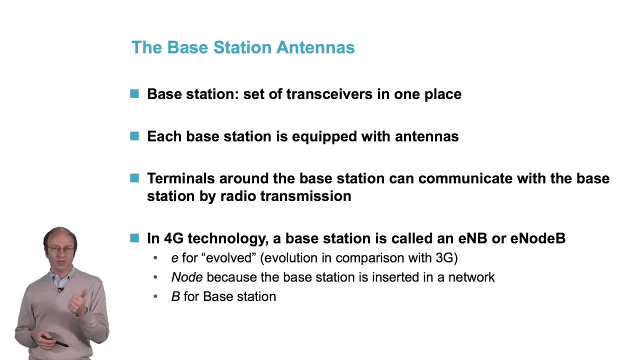 That will enable radio transmission between the terminal, which is also a transceiver, and the network. So we have two things that are very different. So we have two things that are very different: say, a set of transceivers which is located in a place to cover the area around it and 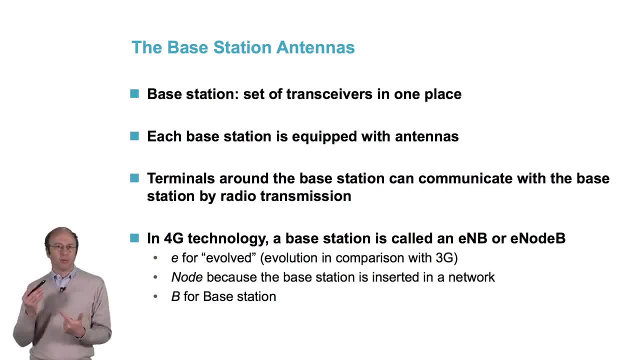 the antenna, which is, so to speak, the tip of the iceberg. the radiating device Terminals around the base station can communicate with the base station by radio transmission. In 4G technology a base station is called an eNodeB- E for evolved to indicate there. 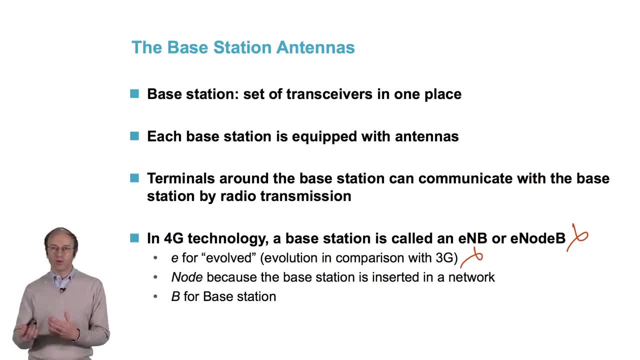 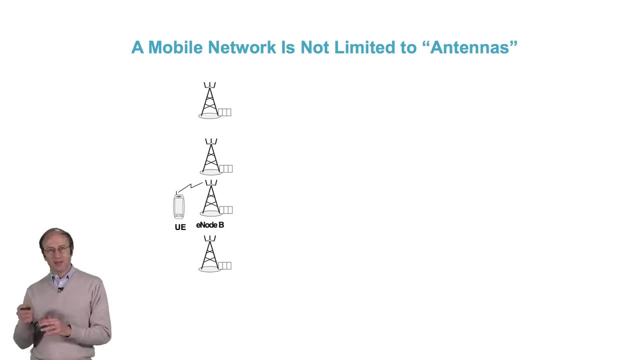 has been an evolution in relation to the previous generation. Node to indicate it's inserted in a network and B for base station. A mobile network isn't limited to eNodes. It's a group of base stations spread out over a territory. The base stations are connected to an IP network deployed by the cell phone operator. 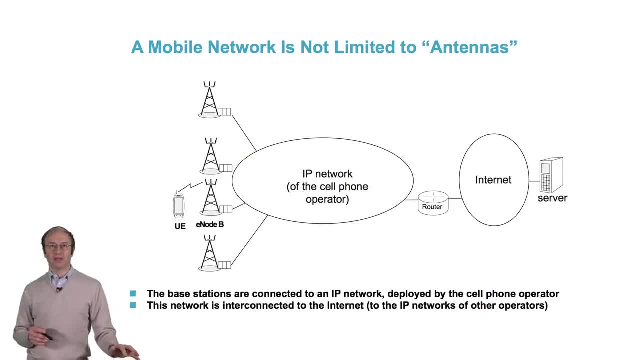 This network is interconnected to the internet, to the IP networks of other operators, via one or several routers. So it's connected to the internet, to the IP networks of other operators via one or several routers. We'll get into the details in other videos. 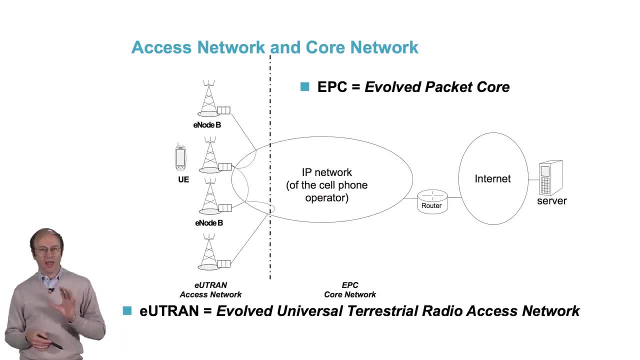 We have two sub-networks: the access network and the core network. The access network is made up of the set of eNodeBs. Because they are connected to the same IP network, they can communicate with each other. In the standard, the access network is called eUTRAN for Evolved Universal Terrestrial Radio.